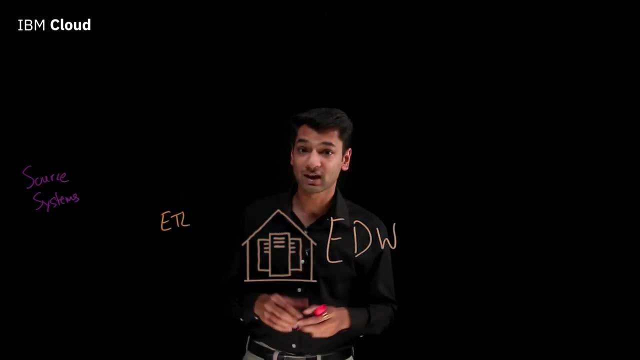 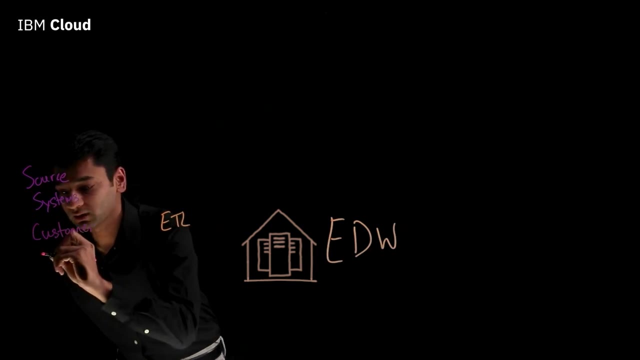 cover a wide variety of business domains, So the data could cover things like Customer data from our CRM. We could have sales data, We could have business customers data data from our ERP systems. you could even have supply chain data, and the list goes. 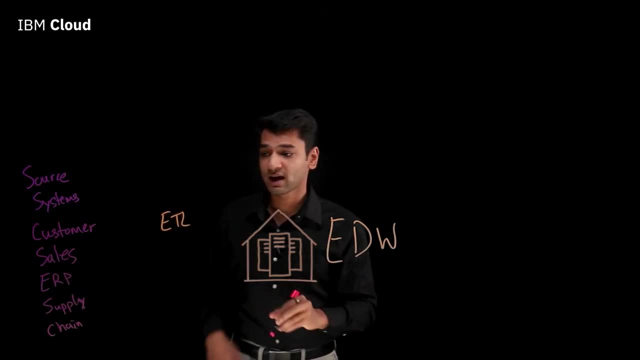 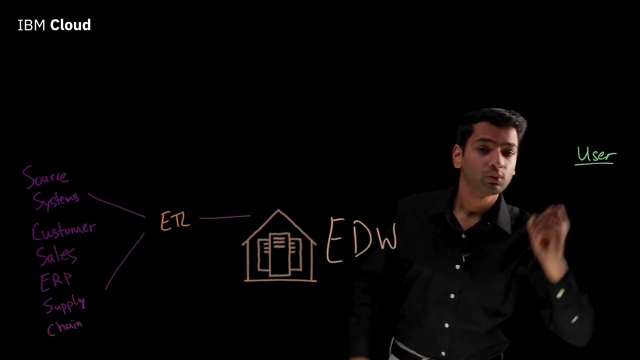 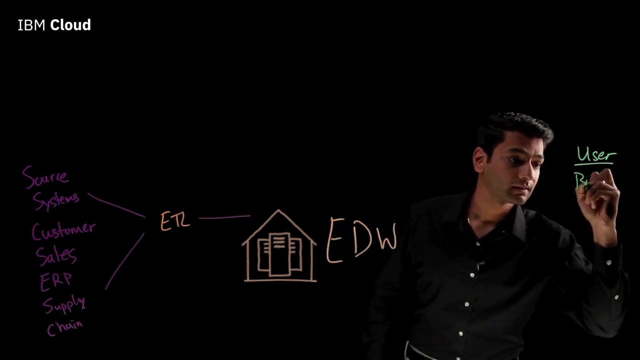 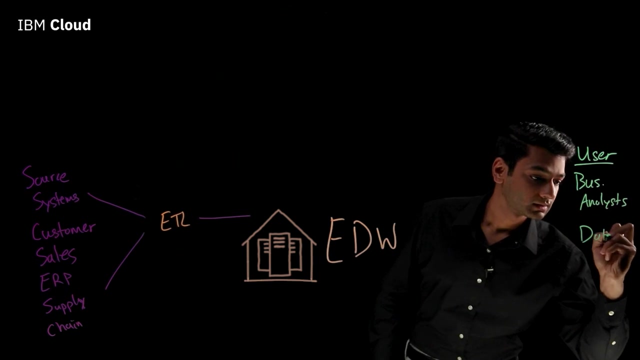 on and on right. so once data has been cleaned, transformed and loaded into our data warehouse, it's now ready for us to expose to our users, who can then start to take it and do analytics and machine learning on these data sets. so who are our users? our users can be folks like business analysts. we can have data. 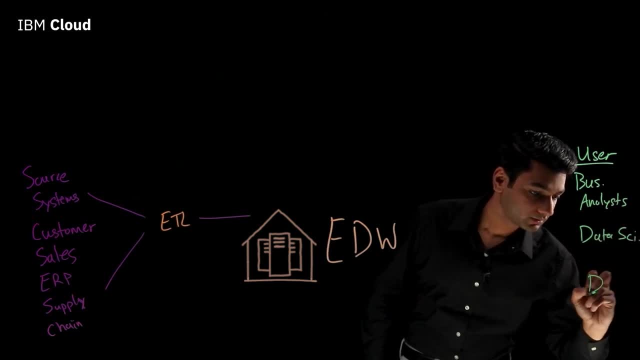 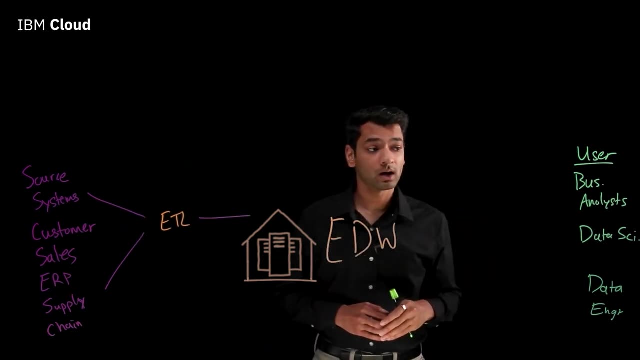 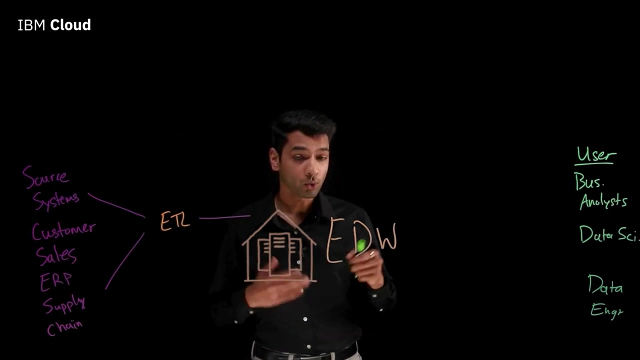 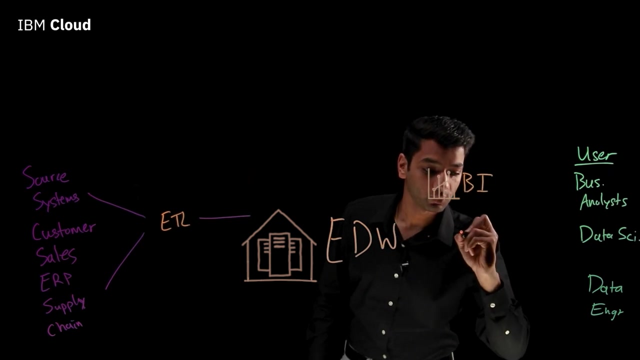 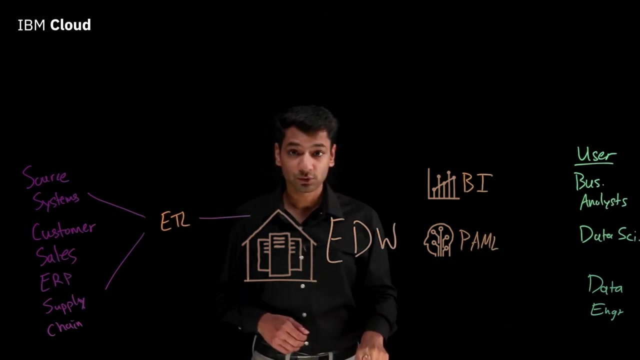 scientists. we could even have data engineers, and these folks can now start leveraging these data sets, either using the built in analytics tools in the data warehouse or using a variety of data, different business intelligence or predictive analytics and machine learning platforms. Okay, so now that we know what an enterprise data warehouse is, let's talk about the different. 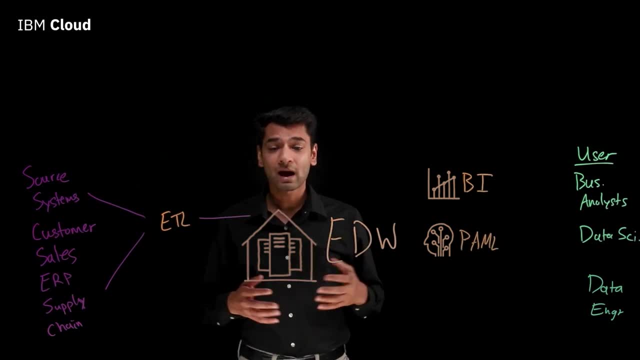 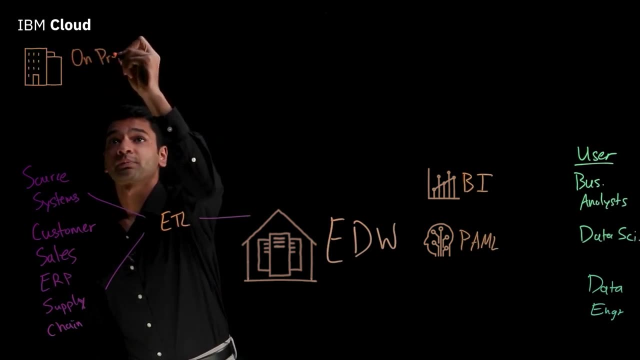 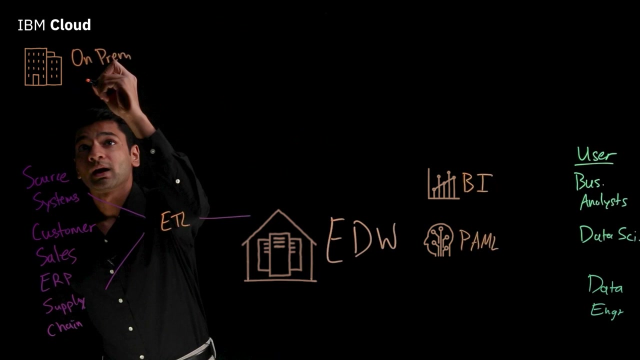 ways in which it can be implemented. So three common ways in which a data warehouse can be deployed. The first way is on-prem. Now a couple different ways in which an on-prem data warehouse can be configured. We could have our data warehouse running on commodity hardware. 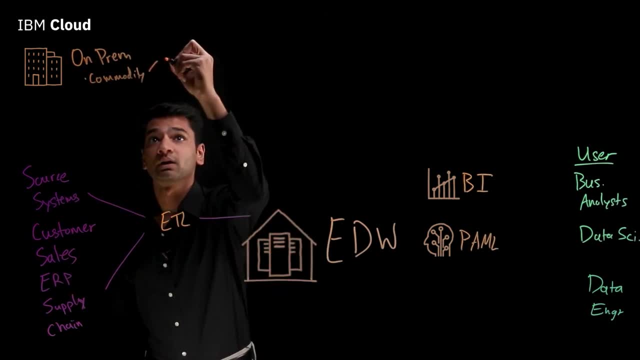 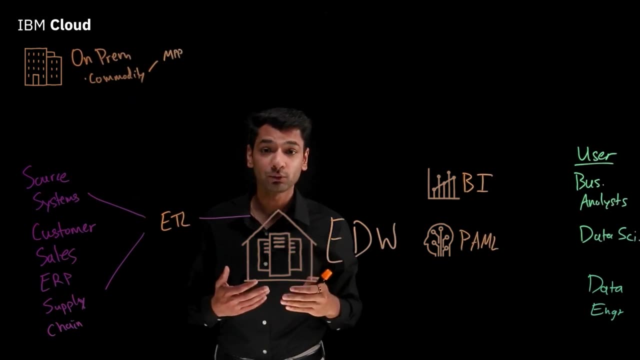 Now this could be set up and structured using either MPP or Massively Parallel Processing Architecture, where we just add more compute nodes as our workload grows, or using SMP or Symmetric Multiprocessing Architecture, Where typically we have a tightly coupled multi-CPU system that shares resources from 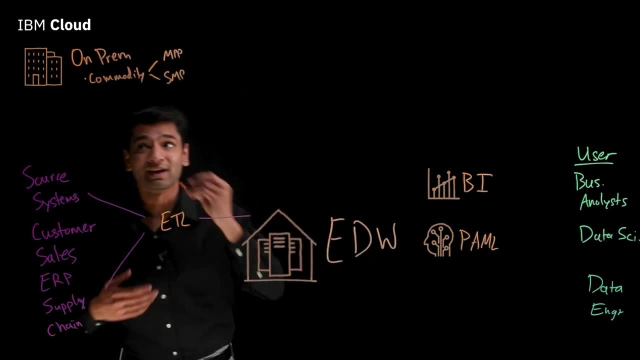 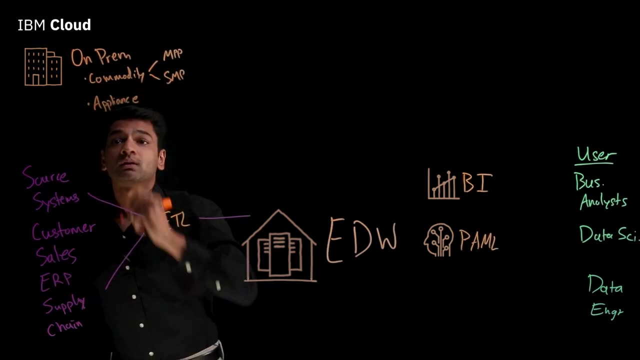 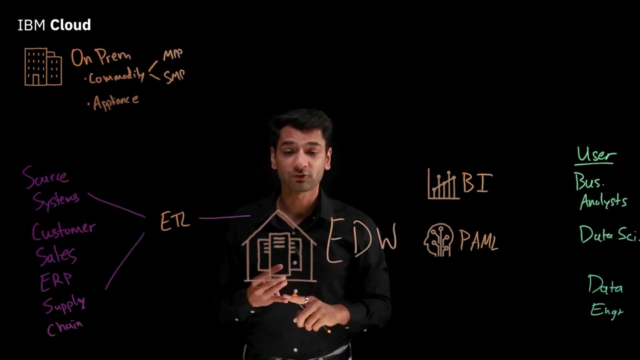 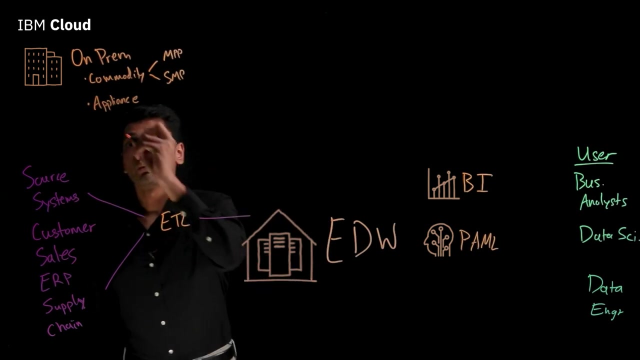 one common operating system. Now, the other way is through a purpose-built appliance format. Now this is typically an integrated stack of CPU memory storage software, all purpose-built and optimized for a data warehouse workload from a single vendor. So what are some of the benefits of having an on-prem data warehouse? 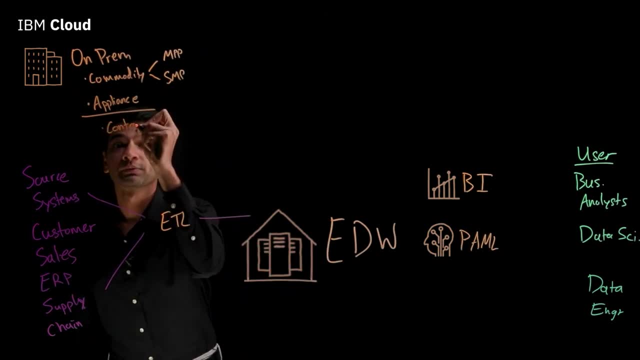 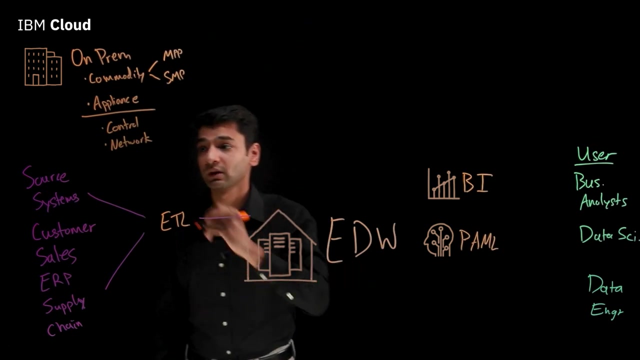 Well, first, you get to maintain complete control over the entire tech stack right. Second, you can leverage your local network speeds and perhaps avoid some bandwidth challenges typically associated with the cloud. You can also leverage high availability, And we can maintain strict governance. 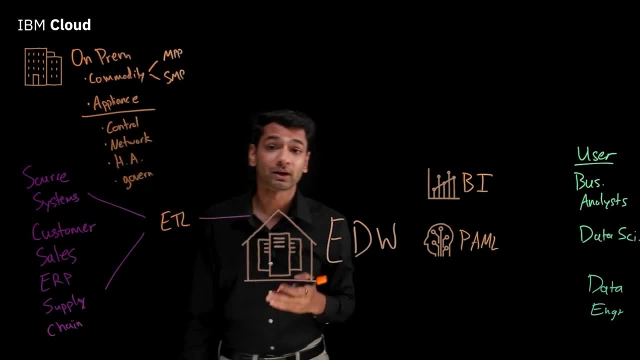 So what are some of the benefits of having an on-prem data warehouse? First, you can leverage strict governance and regulatory compliance. But on the other hand, an on-prem data warehouse does come with an upfront investment and the need for ongoing support and maintenance. 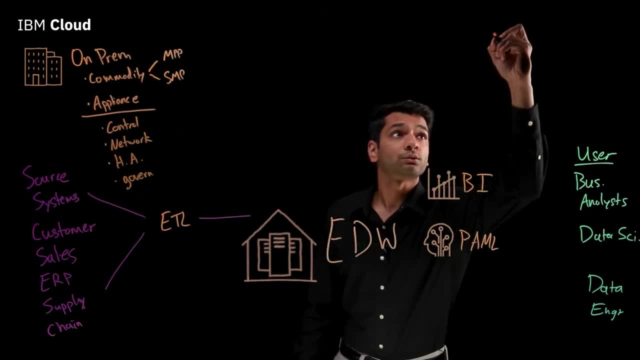 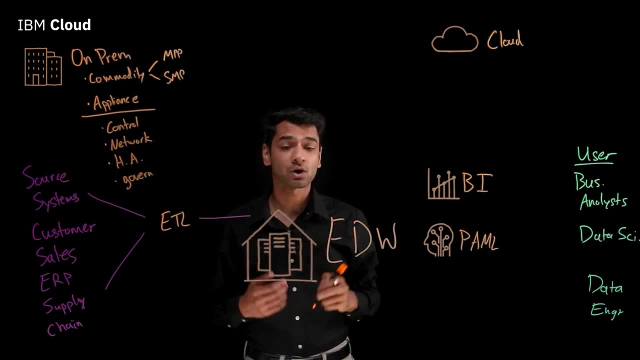 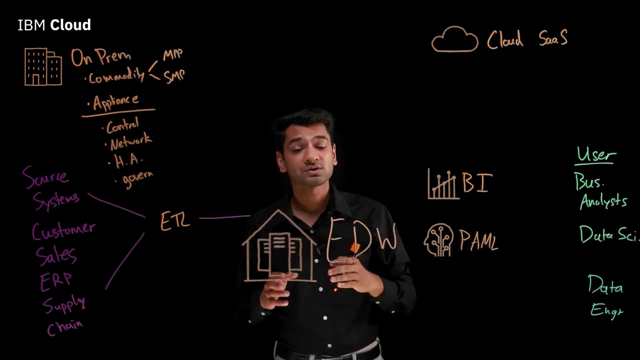 Now, the other way in which a data warehouse can be deployed is through a cloud-based data warehouse, Where our data warehouse is delivered as a managed SaaS offering via the multiple public cloud providers. So moving data warehouses to the cloud is the next frontier for a lot of enterprises. 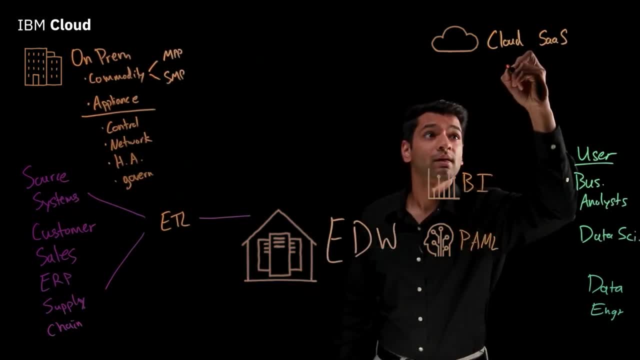 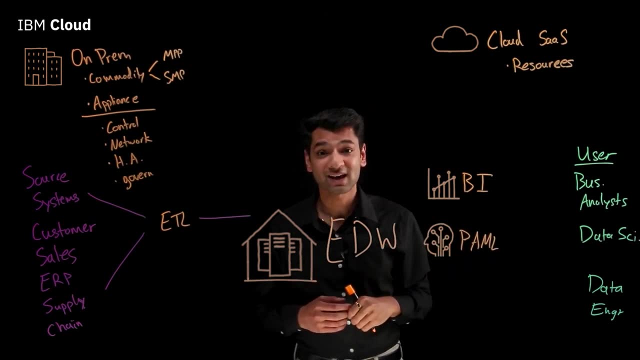 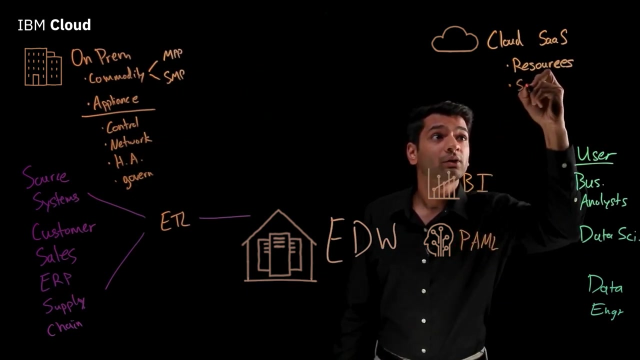 and for valid reasons- right. Some of the benefits include being able to free up resources to focus on other high-value analytics tasks right, instead of just managing systems. Another benefit can also be the ability to scale easily- right, because we don't have to go out and procure new hardware. 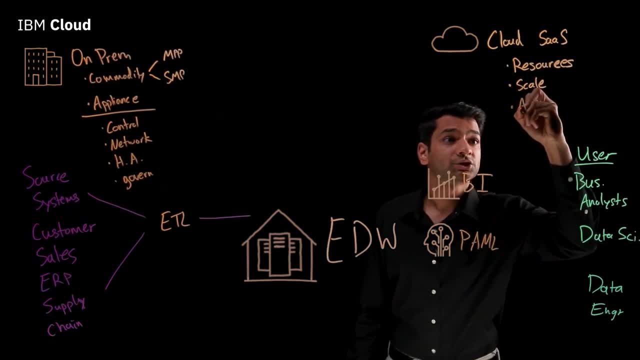 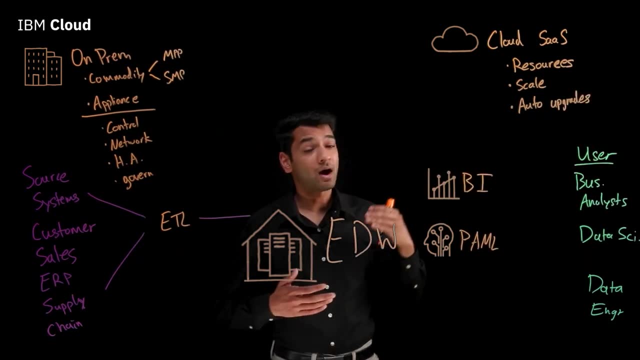 And we get to leverage automatic upgrades right Now. on the other hand, oftentimes a cloud-based data warehouse can take a performance hit due to how it's fine-tuned for that specific workload and there can be some unanticipated high costs due to how cloud data warehouses scale.